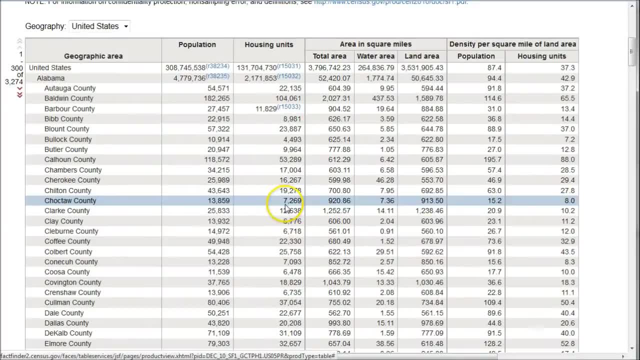 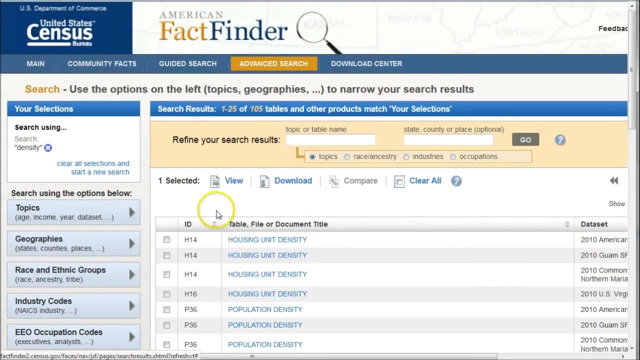 If I scroll down we see it goes from Alabama to Alaska, Multiple states. I'm going to go back to our advanced search here, because that's the data set that I do want, And then I'm just going to click on make sure the one I had is selected and that is selected. 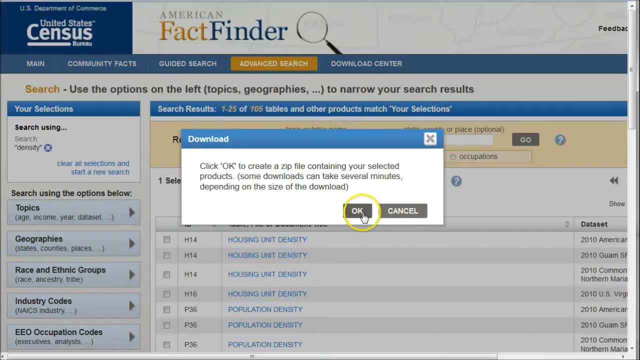 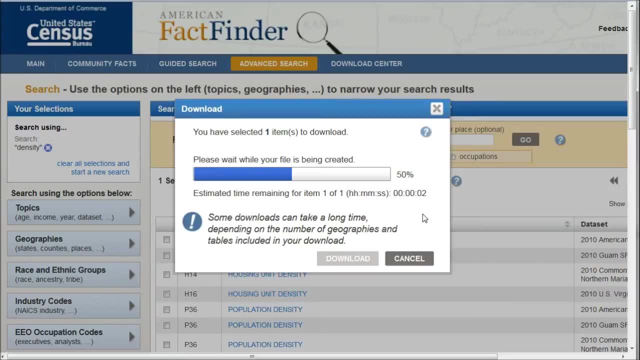 And we're going to click on download And it's going to say, yeah, it may take several minutes, So we'll just click okay, And it's going to go, and sometimes it may take a little while to download this And it will give you an estimated time remaining, that sort of thing. 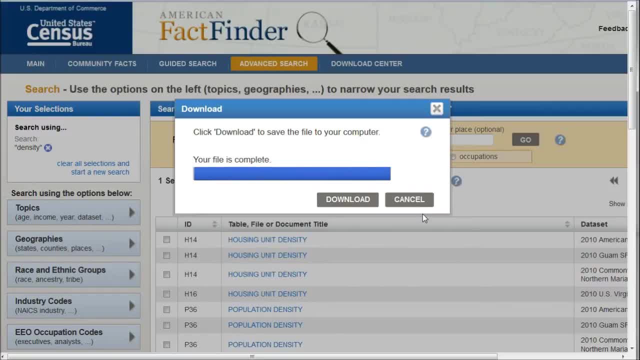 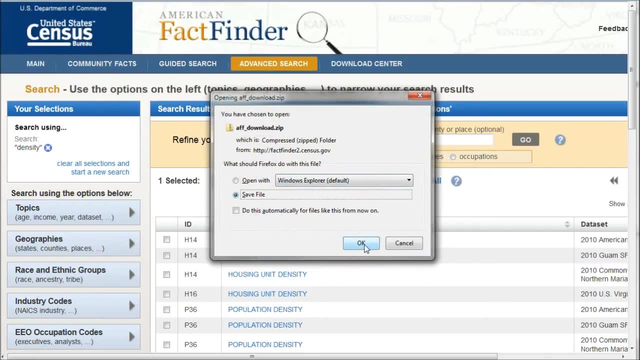 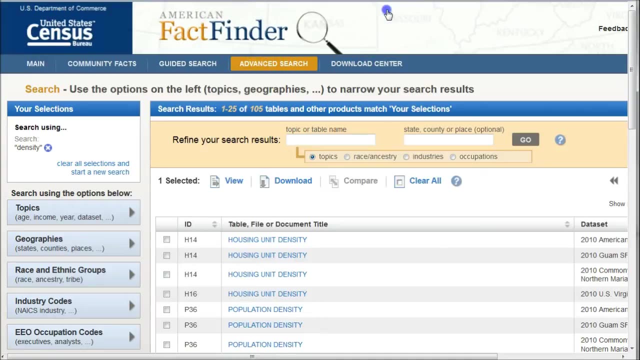 Once your file is complete, all you have to do is click on download And that will open up a zip file. Just save the zip file somewhere on your computer And then, once you open it up, you can see what folder it's in. 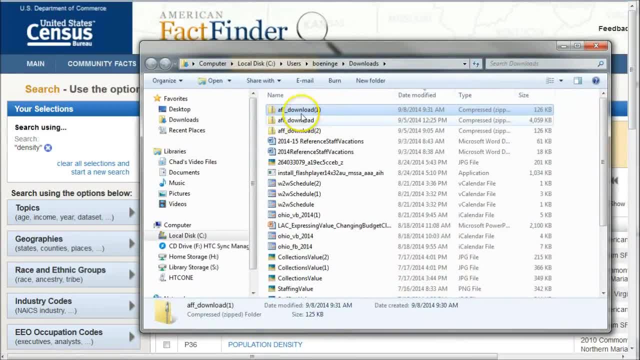 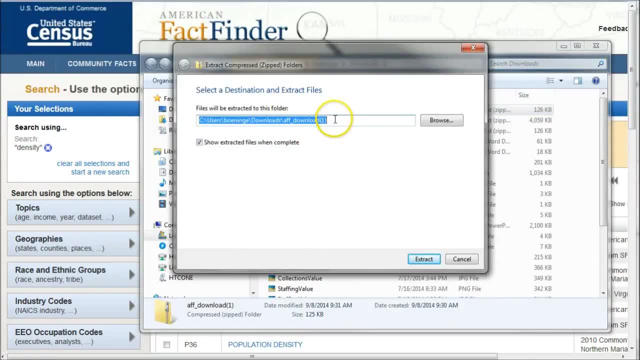 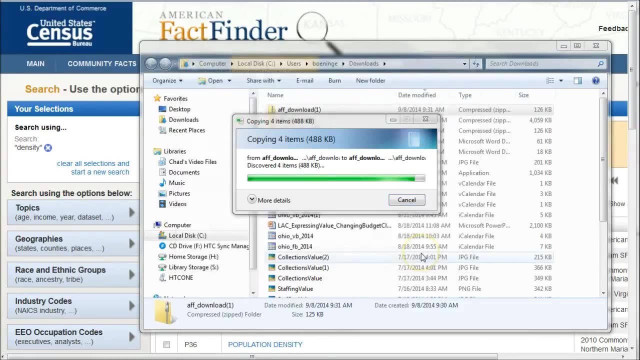 What you'll want to make sure you do is you can go in and extract all your data And we'll just call it census. just download one there. it's fine, We'll extract And then the data set we want is right here. 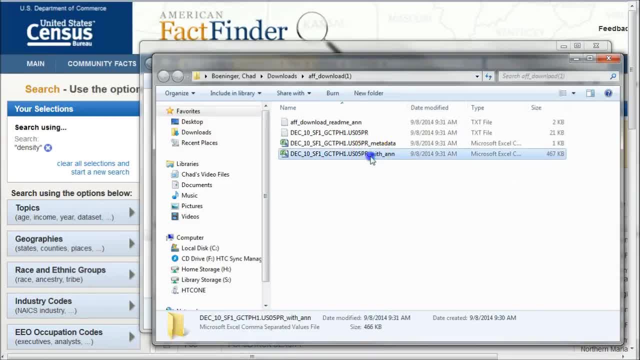 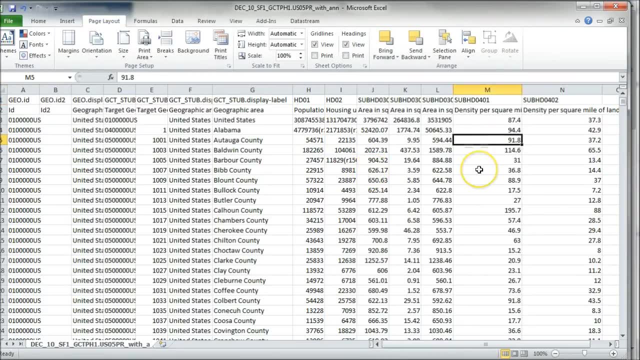 It's called with annotations, I guess is what that means. So we'll open that up in Excel And then here we have our data set in Excel. We can manipulate it however we want to. We can hide tables, that sort of thing. 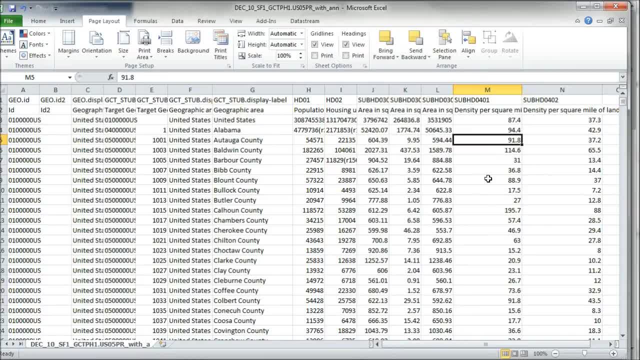 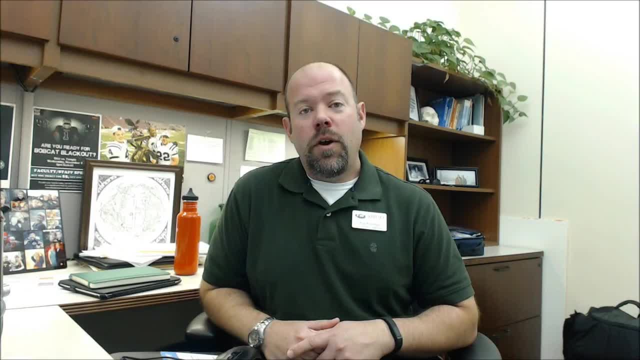 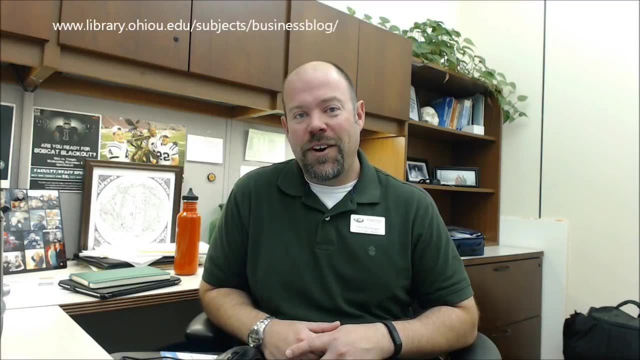 So that's how you find population density in the American Fact Finder using the 2010 decennial census data. Hope this video helped you use the American Fact Finder. Should you need more help, look for the contact link on the business blog. I'll be glad to help you any way I can Take care and have a great day.